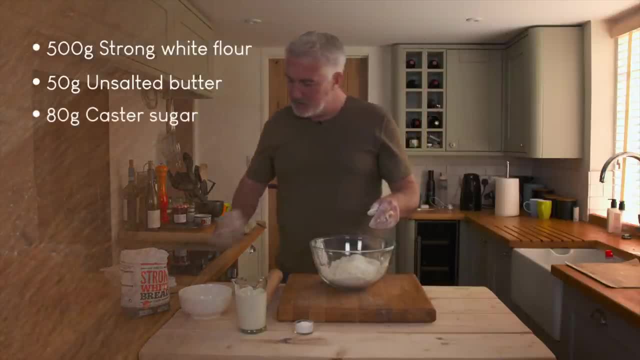 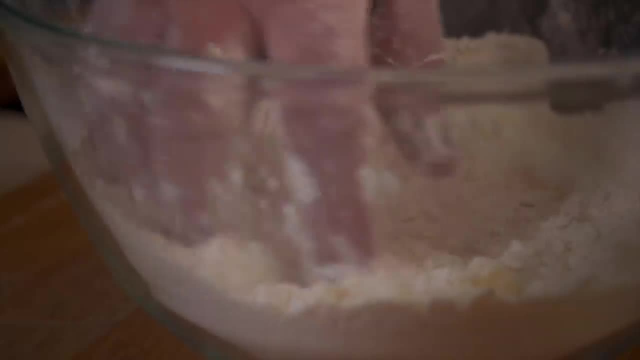 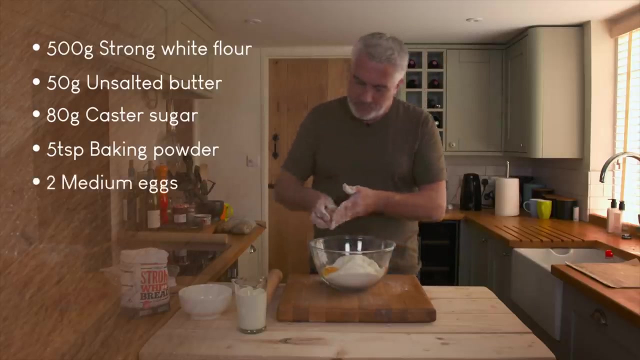 add sugar, caster sugar, straight in. Then I've got my baking powder straight in. Give that a bit of a mix. Perfect: Two eggs straight in. Crack them on the side. What can I do? Clever Right. the next thing to do just gently mix the eggs in And then finally, 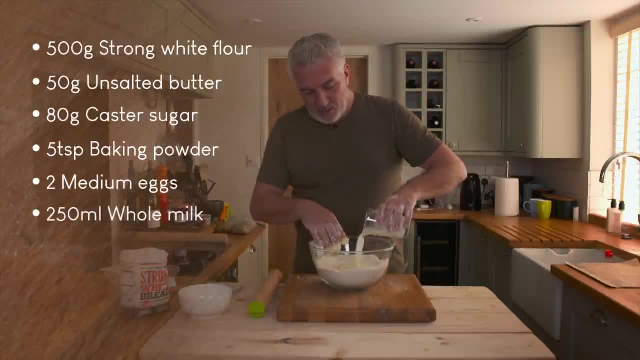 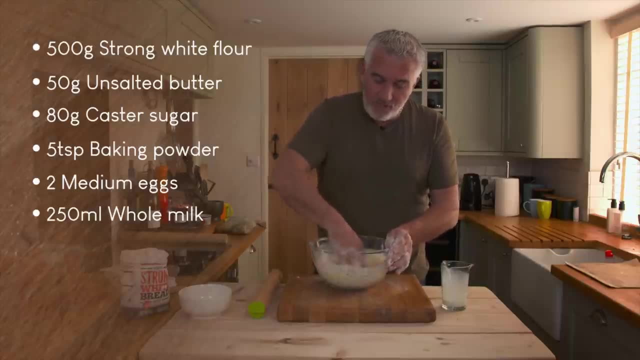 your milk, Whole milk, Hold a little bit back. You just hold it back because I don't know what your flour is like at home. Your flour might be slightly different to mine. Some flours take liquid, some flours don't. So you turn this around, begin to push it. 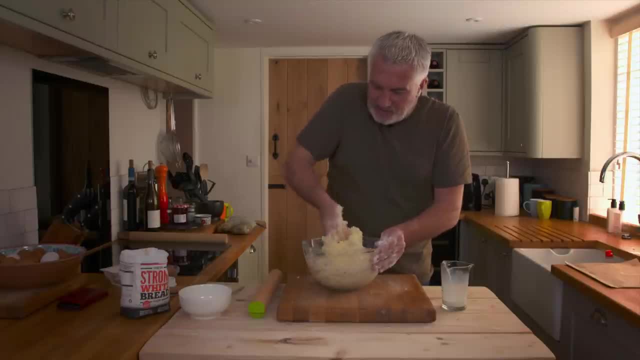 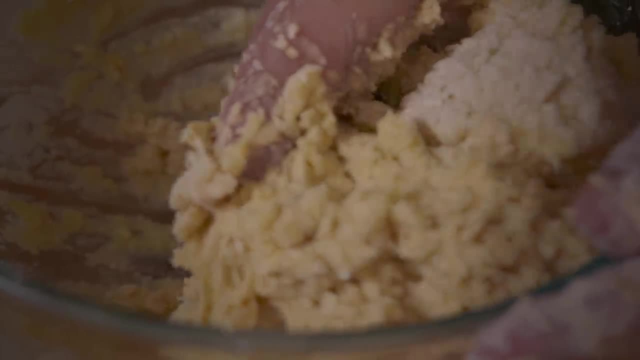 together And you'll see it come together quite nicely into a very soft paste, Very soft dough. Now, at this stage, you have the ball. I'm happy just to leave that little bit of milk to one side, because the flour hasn't done anything. I'm going to add the milk to the 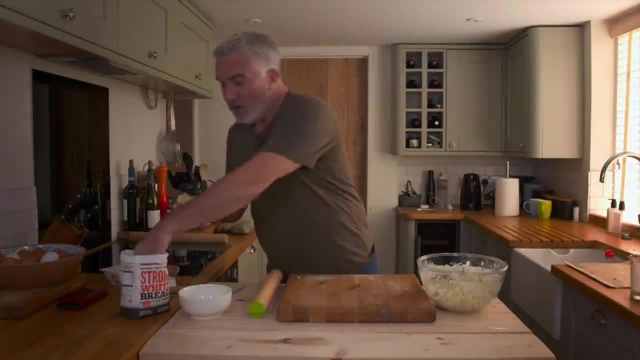 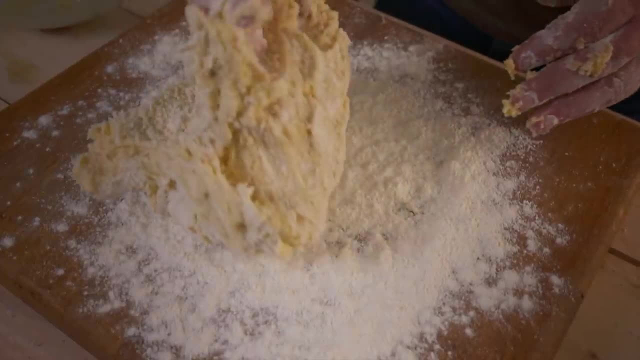 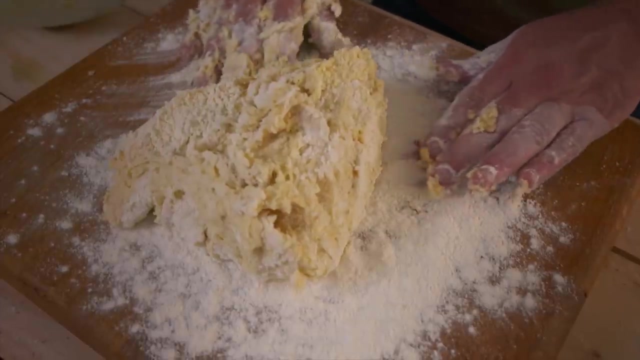 other side because the flour hasn't taken it all. So flour on your surface And then grab your scone mixture. Look how soft that is. How can you tell when it's the right? When it's like that, If it's solid, put more liquid in there. If it's pouring out like 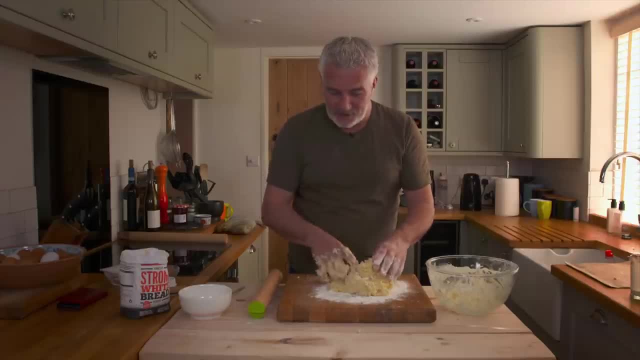 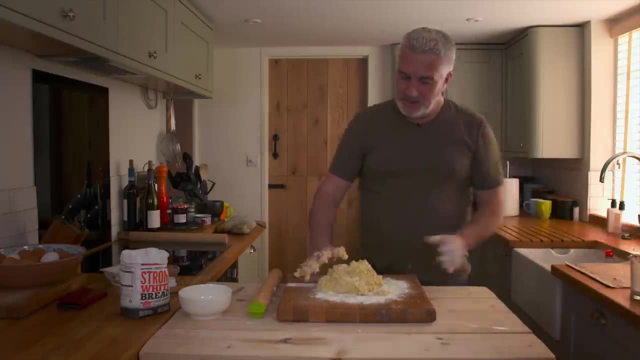 water. you've got too much liquid in there, So you've got to find that balance where it's still quite a lump, but it's still got a little tackiness to it as well. So what you want to do is just basically fold this together. 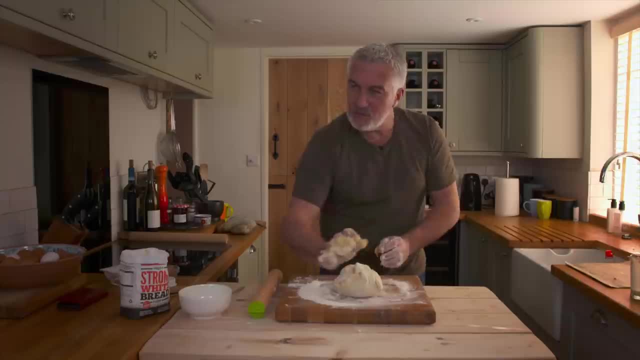 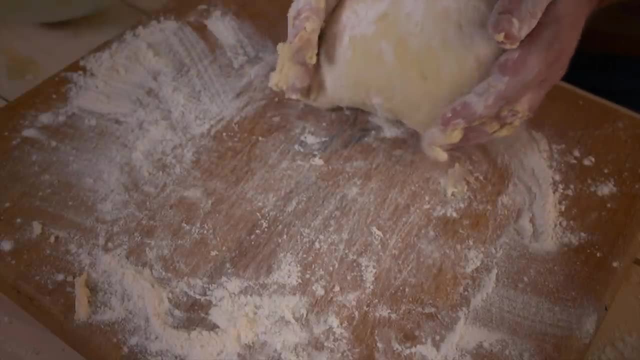 Is that kneading? It's not kneading, it's folding. Kneading is more stretching, Whereas at this stage all I'm doing is incorporating all the ingredients together. So it becomes a little bit more compliant, Just a little bit neater, if you like. 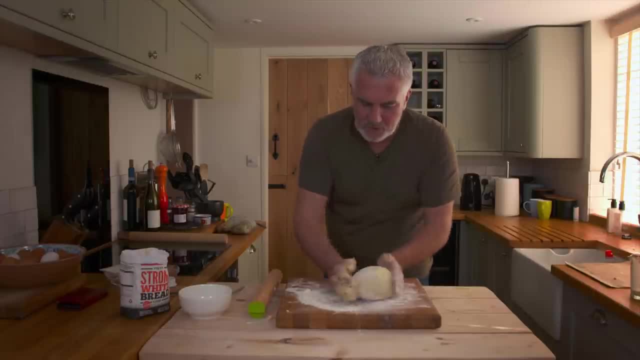 Ten or so movements of that. You don't want to do it too much because it is strong flour. It will bind together and become too gelatinous and therefore won't actually. Well, it'll grow, but it'll just be a little bit gummy on the mouth when you eat your scone. 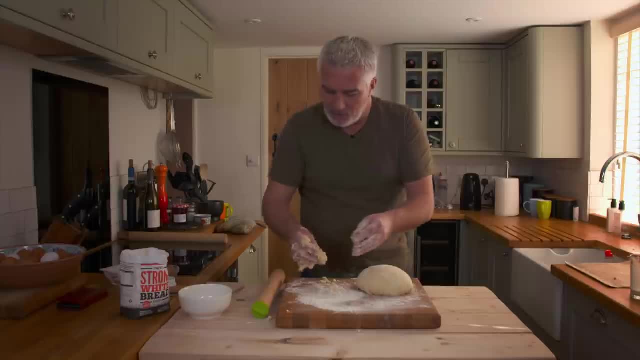 You want it to be quite short. when you eat it, You want it to break apart. You don't want it to be too like chewing gum. you know, Flatten it down And then roll it out from the middle up, middle down, Turn it exactly. 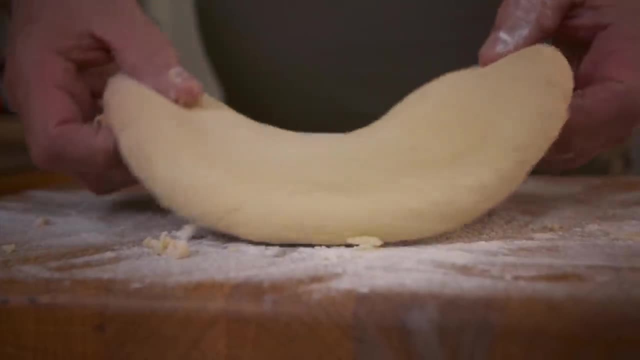 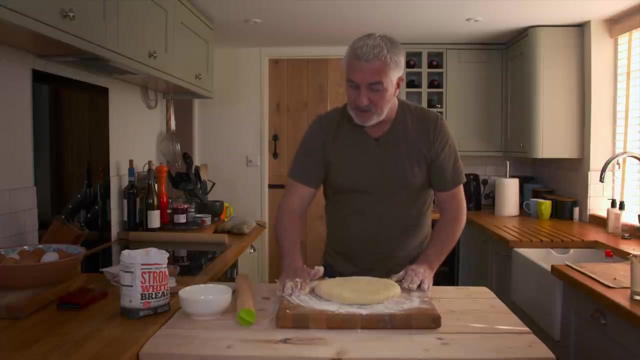 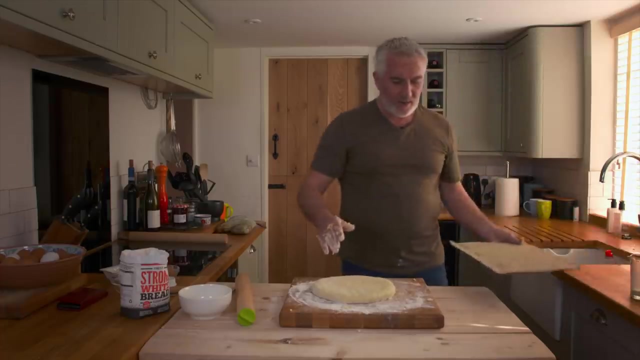 the same again. Keep on turning it because you don't want it to stick. The amount of times I'm seeing people Roll out straight away onto a non-floured surface and it arc-wells itself to the bench. So there's your depth, about an inch. Bring over your tray, Get your scone cutter. 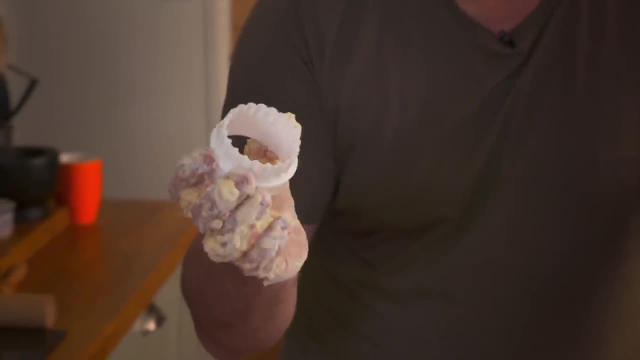 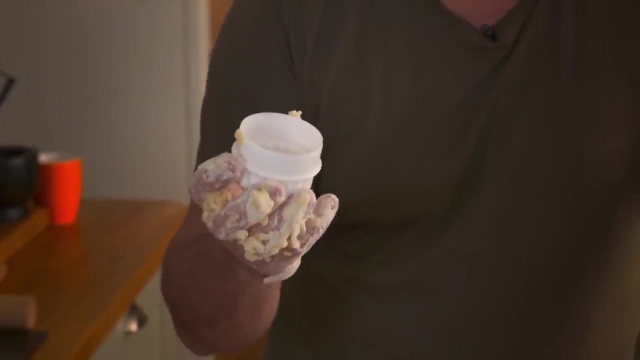 Scone cutter. Very, very posh five-star hotel Me working class lad. There's the difference between the scones. That would be about 20-odd pence in a bakery on High Street. That about £1.50 in a five-star hotel in London. That's the difference between the two. 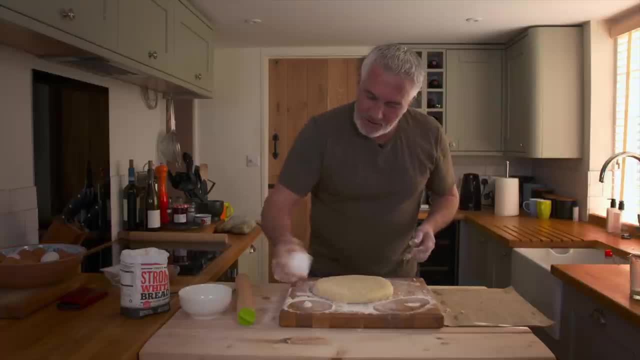 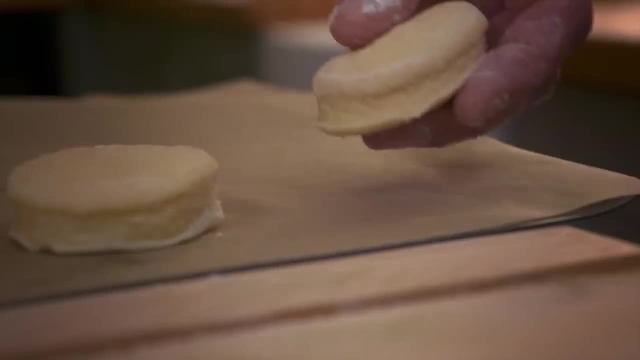 Okay, Turn your cutter in a little bit of flour, because it just helps release it, And then place them onto your tray And I'm relaxing the dough. The last thing I do is roll it out too much on a sticky surface. cut it and it goes. 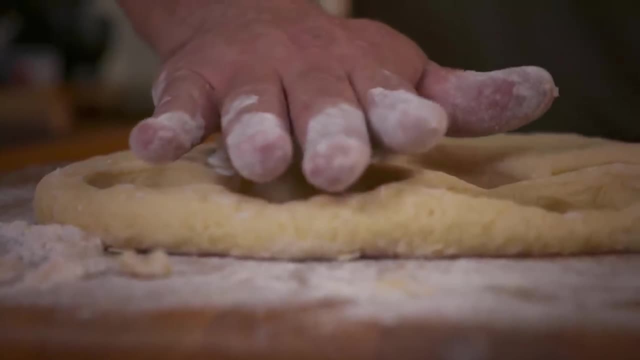 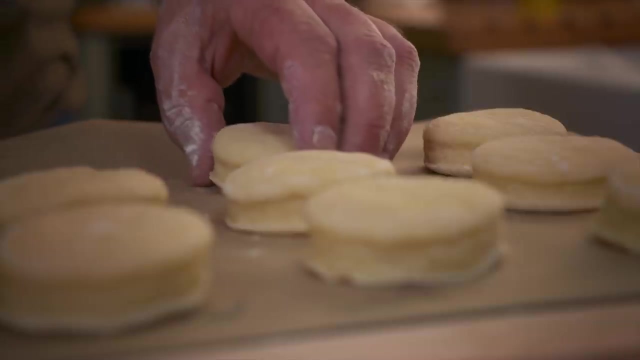 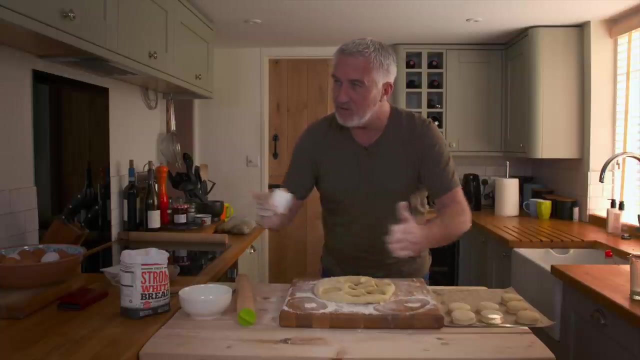 I'm relaxing it all the time so it keeps its shape. How are you doing that? By keeping it plenty of flour underneath it. it prevents it from shrinking because it's relaxing at the moment. So if I cut that, stays that shape. If I stretch it out and cut it, it'll go boop because it's trying. 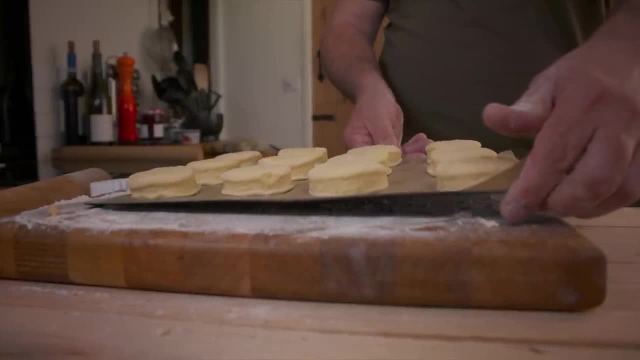 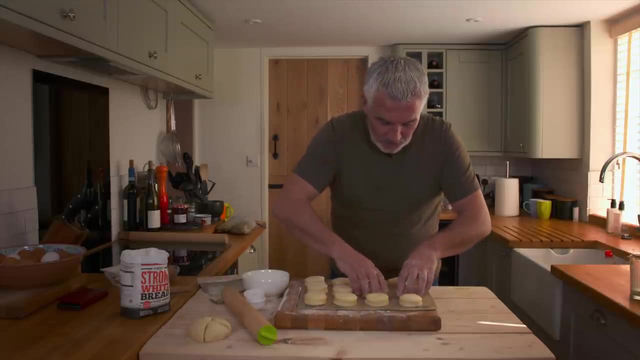 to contract again. There's your scones, which are beginning to rise already. The baking powder in here will always be active. now Your oven's nice and hot, Just making sure they can move. They're nice and neat and round. 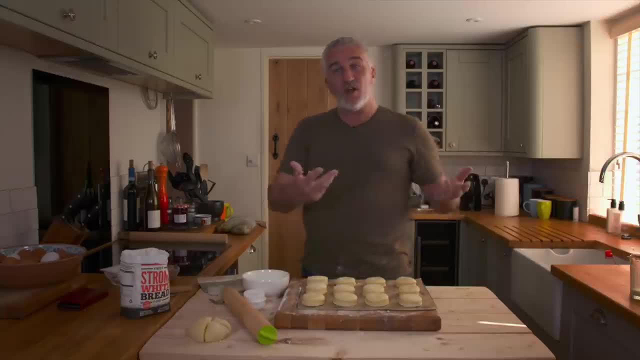 How does baking powder work? Baking powder basically produces carbon dioxide. The baking powder in there reacts with the milk, the acid, and that creates carbon dioxide and that begins to grow. It has a finite life. It's not going to last for hours, So you've got a window of about probably an hour or 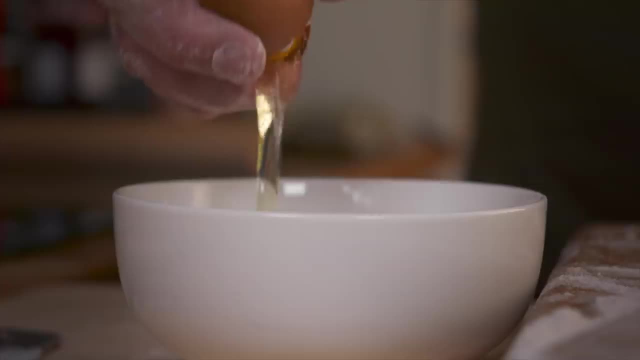 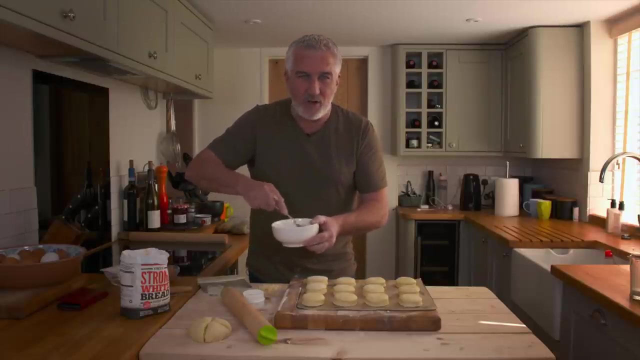 two to actually use it before it starts losing its power. So again, egg straight in the bowl, Literally just an egg in a bowl. Try not to add any milk because it dilutes that color and you want that beautiful golden brown color when.